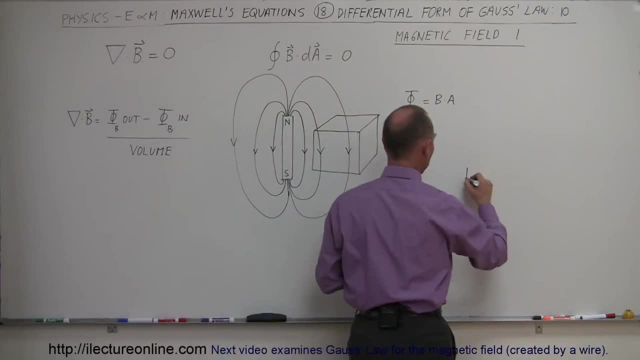 For example, if we take this magnet and I'll draw a little curve smaller like this, so let's say we have a north pole and a south pole, like this, and we draw a gaussian surface around it, now you have what we would call a source of magnetic field lines. but 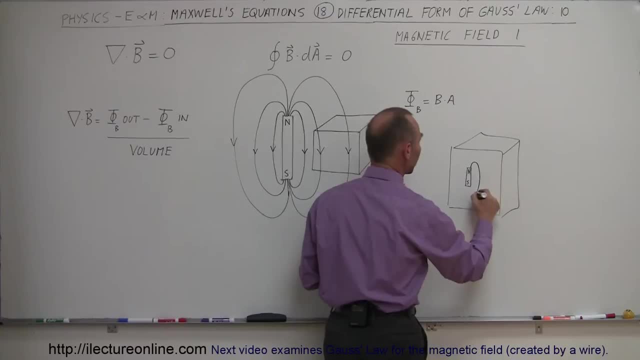 what happens is that all the field lines will start from the north, go down to the south, like this, north to south, like this, and i'm just drawing one side of it, north to south, like this. you can see that because of this source, you have some lines coming out of the surface and then coming. 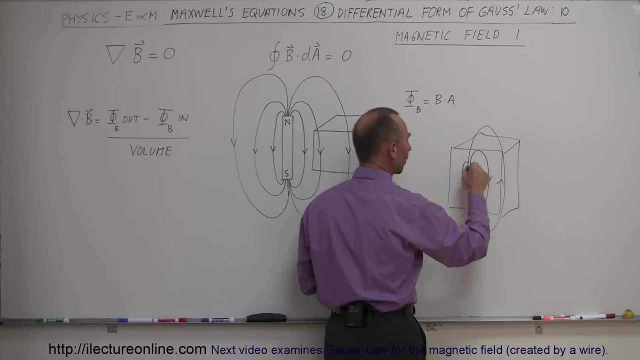 back into the surface and what? what we can then conclude- and let me draw the other side as well. there we go. what we can then conclude is that if we do this over the entire surface- when i say do this, meaning take the surface integral of the strength of the b field, the magnetic field, 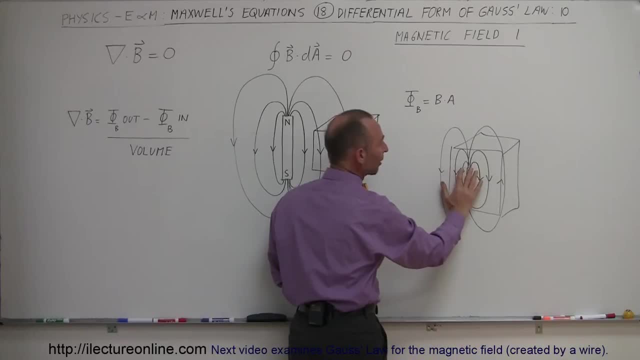 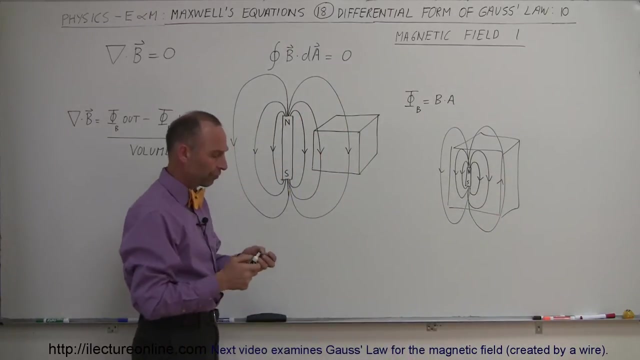 times the surface, then we have an equal amount of field lines going out of the surface, going into the surface, and they end up casting each other out. and so, therefore, again, since all field lines end up returning back to the source, when we do a gaussian surface integral, we end up with a zero result. and so, therefore, it was concluded that 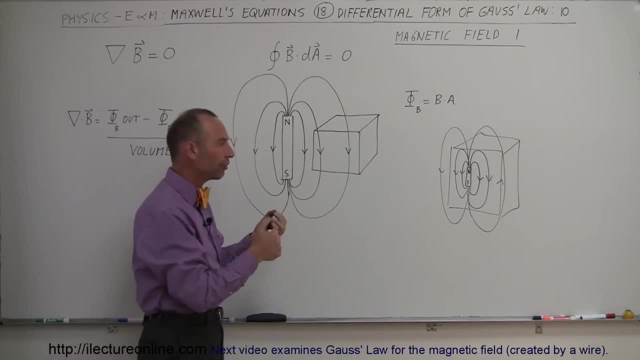 there was no single north pole or single south pole in the universe. that could cause a net excess of field lines going out versus field lines coming back in. so in magnetic fields you always have the same number of field lines going out of the source as coming back in to the source on the other side. 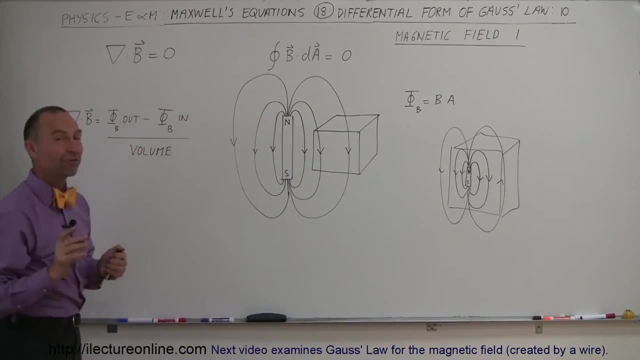 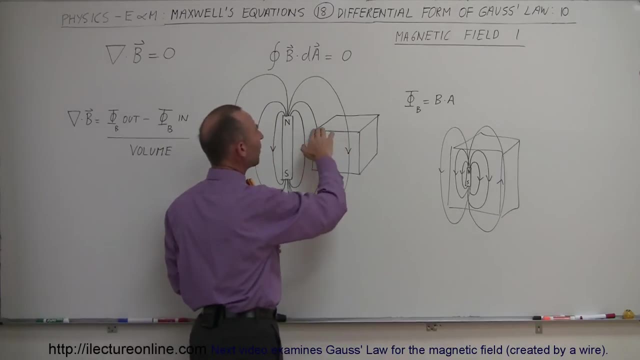 but if we take a look at the differential form of gauss's law for magnetism, it seems to make a lot more sense, and here's the reason why, again, what we can do here is figure out how much flux is going into the cube and how much. 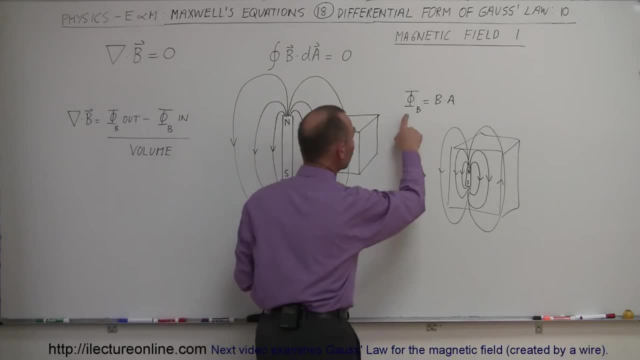 flux is coming out of the cube and remember, flux is equal to the strength of magnetic field times the surface area. so that indicates how much flux is going into the cube and how much flux is going out of the cube. and what gauss's law says is that the divergence of the magnetic field is equal to. 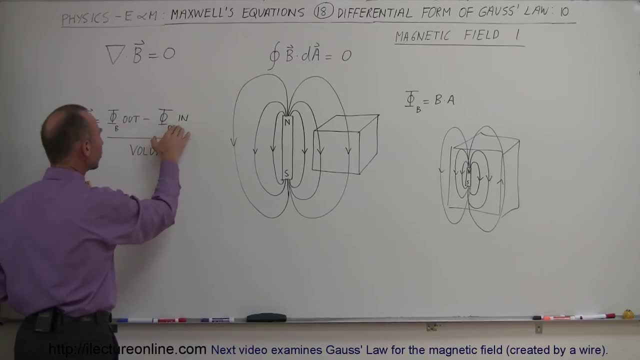 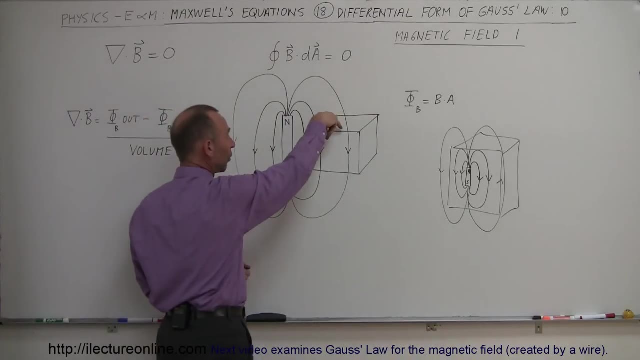 the amount of flux coming out of the cube minus the amount of flux coming in the cube divided by the volume of the cube. but here, by simply looking at the drawing, you realize that in this case we have two field lines going in, two field lines coming out, the.